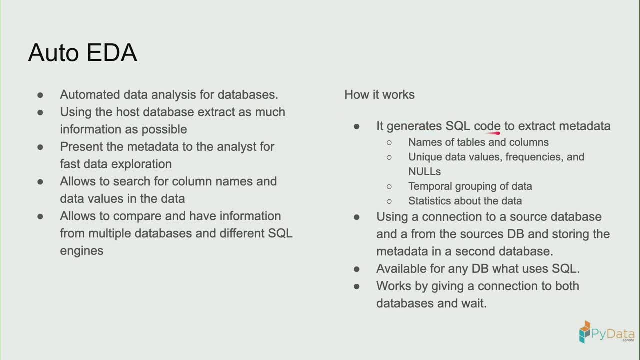 So how it works. Basically, the library or the script auto-generates SQL code and extracts column names, table names, features like distinct values, nulls in the data set, Temporal code, Temporal grouping of the data when you have timestamps and some statistics. 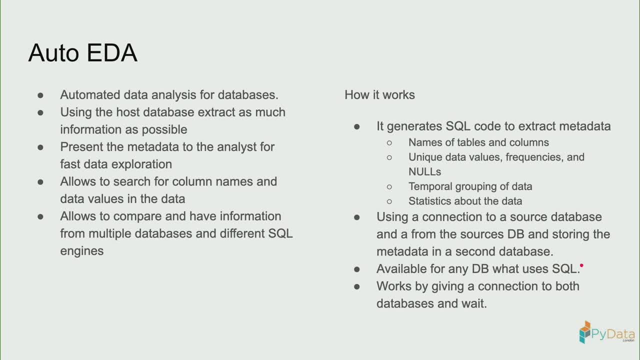 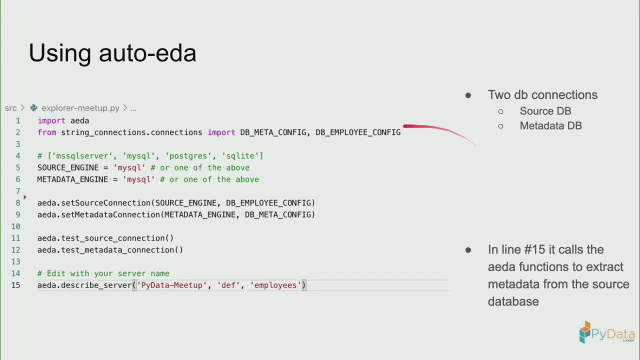 You just need to provide a connection to your source and a connection to your metadata database. This is a simple configuration. Basically, you import the library and you basically pass the two connections, Or you import the two connections And you just need to configure it here. 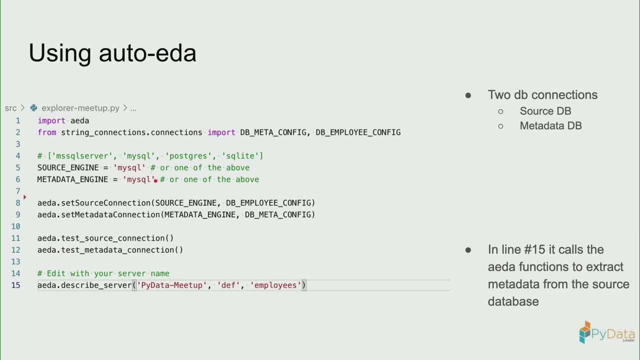 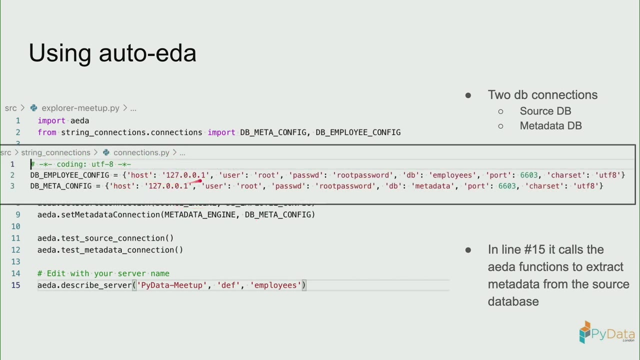 Where is the? You specify the server, You specify what type of engine. a MySQL SQL server is working pretty well, Postgres as well, and SQLite, And basically just these connections are where the server lives: the root, the password. 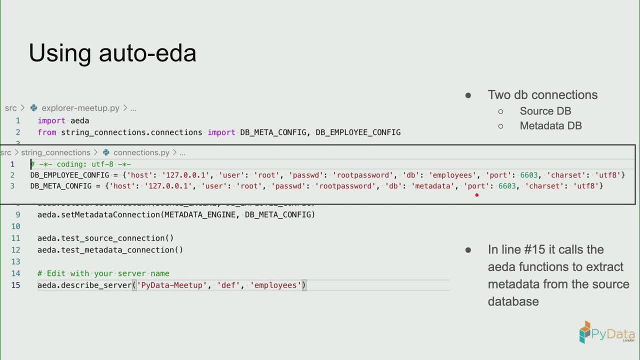 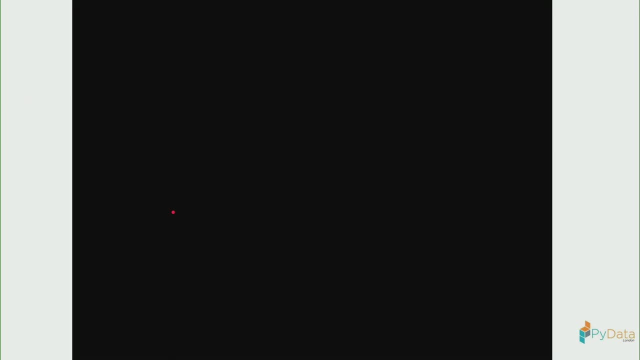 I'm using for this example the employee's database from MySQL, So in line 15.. Basically, it calls, It calls the library using these connections. You just pass these connections, You have your data in your databases And we will see a wee example of this. 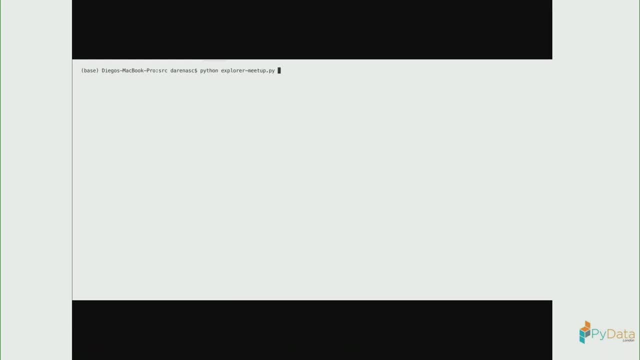 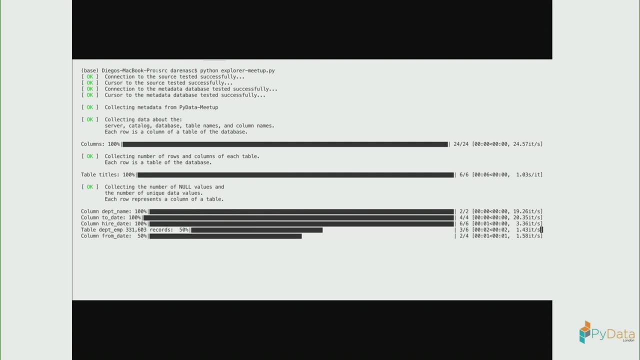 So, basically, I'm calling this explorer, I call it mid-app. It makes the connection, reads first the columns of the tables, then reads the tables And it starts extracting information from the columns: Distinct values, nulls And then the temporal data. it groups the temporal data automatically. 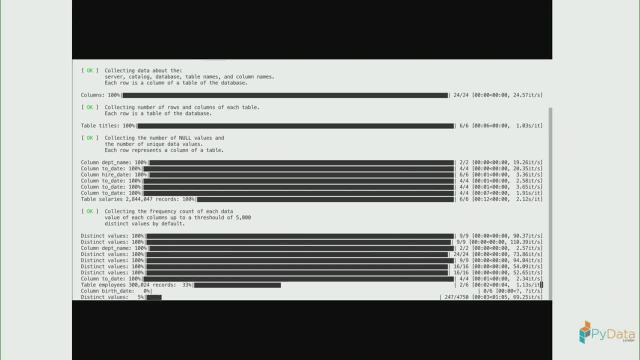 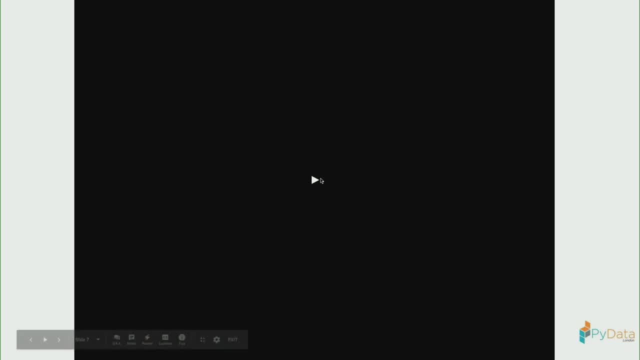 So at the end of the process you just leave this running. At the end of the process you will have a database that you can query and puts any tool that you want to visualize. So the backend, or the metadata database, will have six tables. 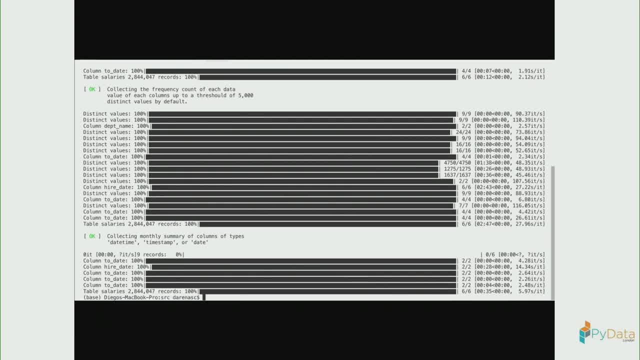 At the moment one for tables columns. You can see the code in the repository- I will share it at the end of the presentation- And basically it goes through all the kind of metadata you would like to analyze And you have everything in one place.